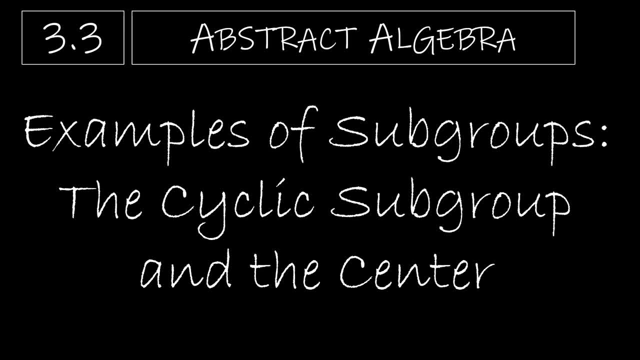 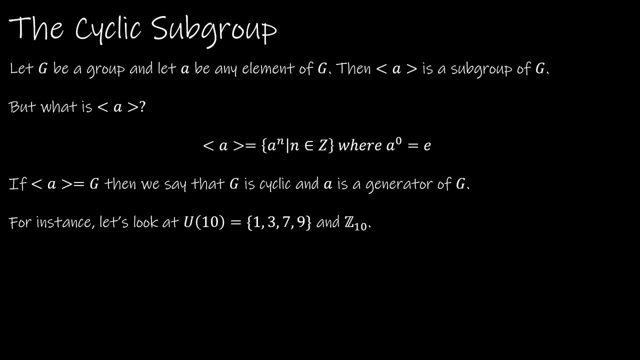 In the last video for chapter 3, we're going to take a look at two more examples of subgroups, which include the cyclic subgroup and the center. The first subgroup we want to look at is the cyclic subgroup. It kind of seems silly to study the cyclic subgroup right now because we haven't talked about cyclic groups. We are going to dive deeper into that in our next chapter, but let's go ahead and get a nice little preview. So if G is a group and A is an element of G, then we say that this means the subgroup generated by A is a subgroup of G. So essentially we're saying that A is a generator and we're going to take A to every power. And what's going to happen in a cyclic subgroup is it's eventually going to get back to E, which is a to the zero power. So let's take a look at what I mean by that, because it's going to make a lot more sense when we look at an example. We already know the group U10. So remember, the group U10 is elements that are less than 10, but relatively prime to 10. And the operation is matrix multiple, I'm sorry, not matrix, is modular multiplication. So essentially, we're saying that one would be one to the zero, one to the first, one to the second, and so on and so on. Now, what's going to happen when I take one to the zero and one to the first and one to the second? Well, the only thing I'm going to get is one, which is, in fact, the identity. So while one, the subgroup 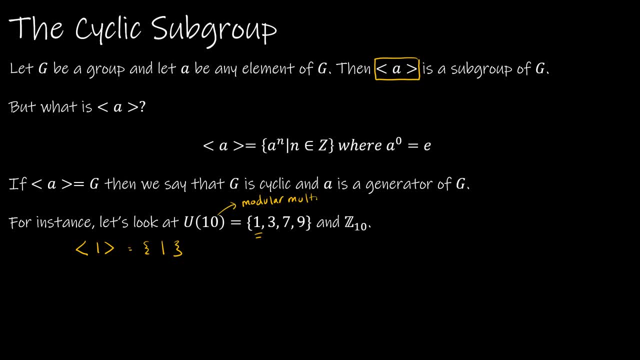 generated by one, is, in fact, a subgroup, it doesn't generate every member of the group. So if the element generates every element of the group, we say that the group itself is cyclic 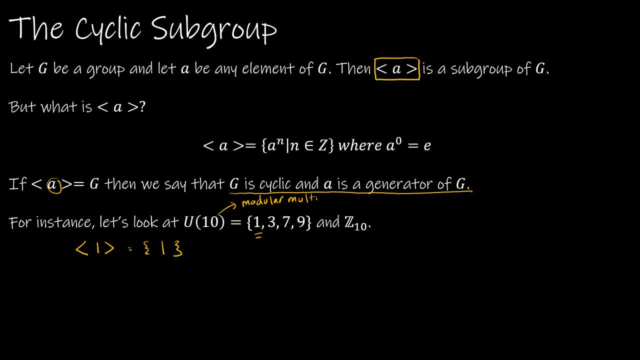 and has a generator of A. So let's keep looking at U10 to see if there are, if in fact, this is a cyclic group, and if they have any generators. So let's look at 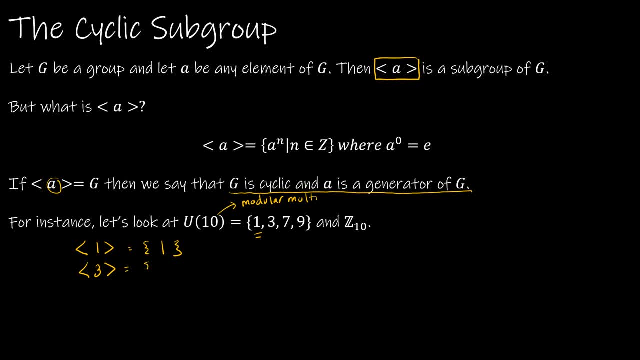 three. Remember, three would be three to the zero, three to the first, three to the second, which is nine, three to the third, which is 27, but we're mod 10. So 27 is, actually, seven. And then if I go to the next one, three to the fourth, it's actually going to bring me back to one. So as we can see, U10 is, in fact, a cyclic group that is generated by 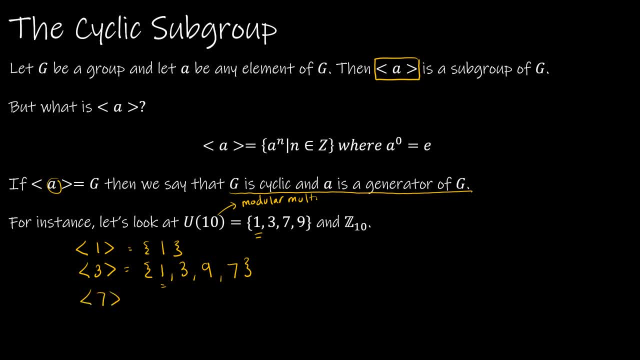 three. Well, what about seven? Because a group can be generated by more than one element. 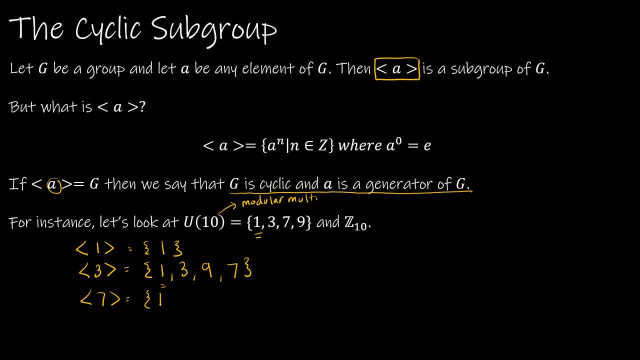 Looking at seven, I have seven to the zero, seven to the first, seven squared is 49, which is just nine, seven to the third is 243, which is three, and we would end up back at one. So seven does generate every element of the set. 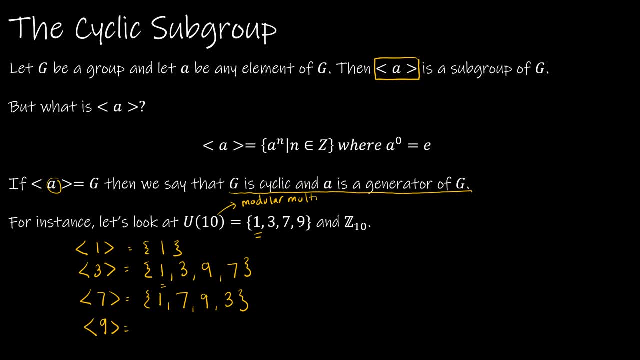 If I look at nine, nine to the zero is one, nine to the first is nine, nine squared is 81, which is one. So one generates only one, nine generates one in nine. Those are both subgroups. Oops. Wow, 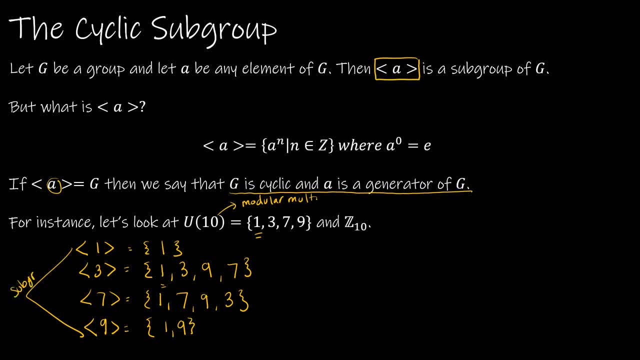 let me just try that again. These are both subgroups, as are three and the, sorry, the groups generated by three and seven. So all four of these are subgroups. They all include the identity. 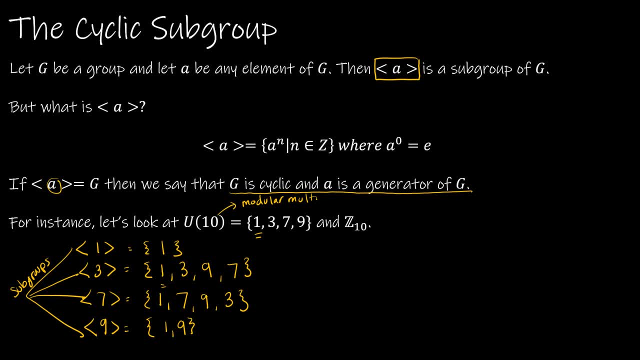 the um the subgroup tests would be met i'm not going to go through that test with you but they would all be met obviously closed and so forth but we can also then say that specific to three and seven that three and seven generate the entire group now let's look at z10 so z10 is a little 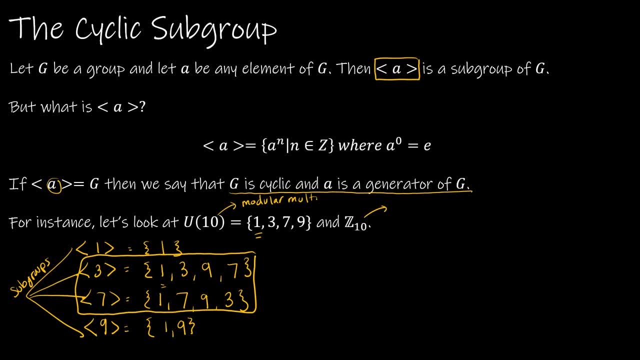 bit different because this operation is addition so it's it's modular addition so it's going to be a little bit different so instead of 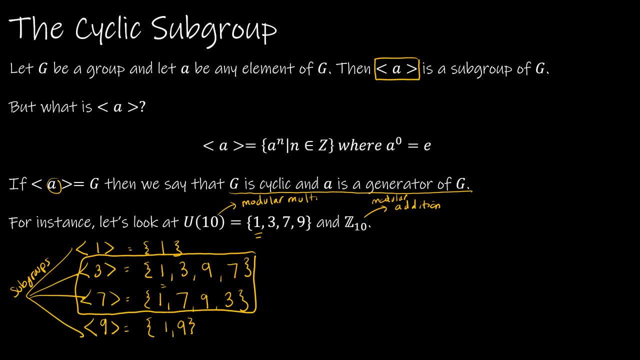 one squared two squared and so forth we would be looking at multiplying instead so instead of powers from multiplying this goes back to multiplicative notation versus additive notation 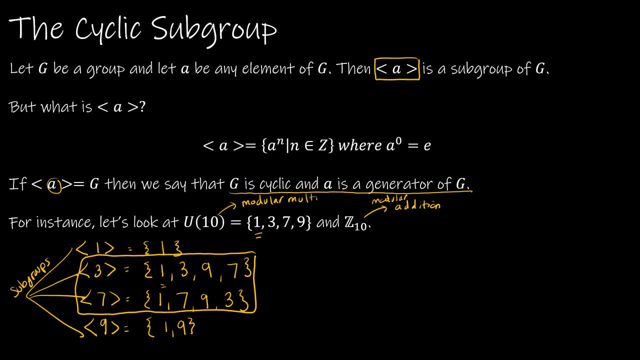 that we talked about in chapter two so what can i say about one and i'm not going to go through all of the elements but 1 would just be 1 times 0 whoops 1 times 1 1 times 2 1 times 3 1 times 4 and so on so i'm going to get all of the elements so one is going to generate the entire set. Well, what about two? Two is going to give me two times zero, two times one, two times two, two times three, two times four, two times five. That's back to the identity. So one does generate the entire set, whereas two would generate only the even values of our set. Again, both are subgroups, but we only have certain generators. So we didn't go through all of the values in Z10, but we know at least one does generate every value in the set. 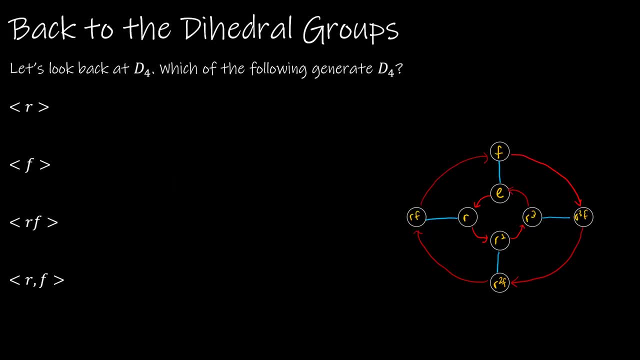 We've spent some time in this class talking about the dihedral groups. So let's look back at D4 and talk about if D4 has any generators. And we're not going to go through all of the generators, but I do want to talk about what the dihedral groups are. So let's look back at D4 and talk about what each element does generate. So if I look at R, remember R would be R to the zero, R to the first, R squared, R cubed, and then R to the fourth in D4 would go back to the beginning. 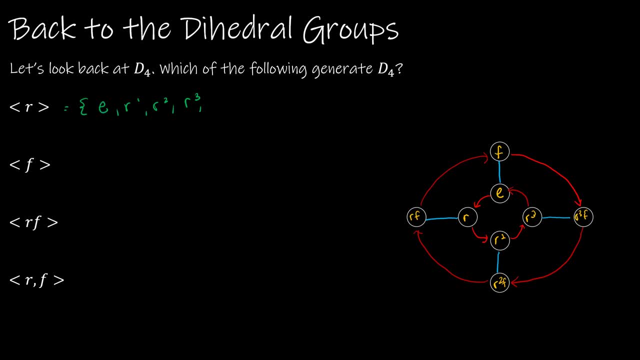 So R to the zero, we call the identity. Then R to the first, we just call R, 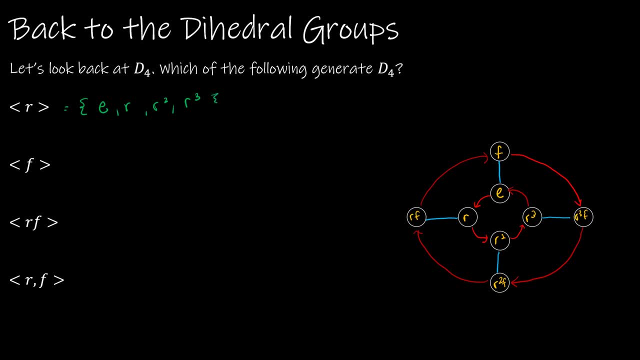 and then R squared, R cubed. So we can see that really we're looking at the elements in the center, 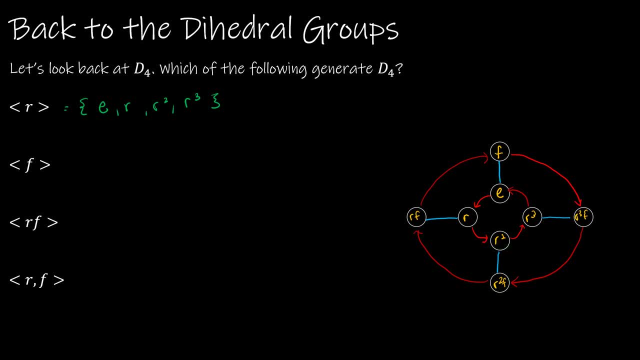 of our Cayley graph. What about F? Well, F would just be not flipping at all, 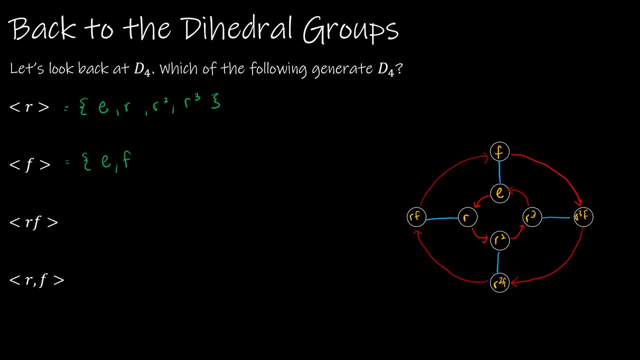 which is the identity, and then flipping. And then if I flip twice, what happens? Well, I go from E to F on a flip, and then I would go back to E again. So that is a subgroup, 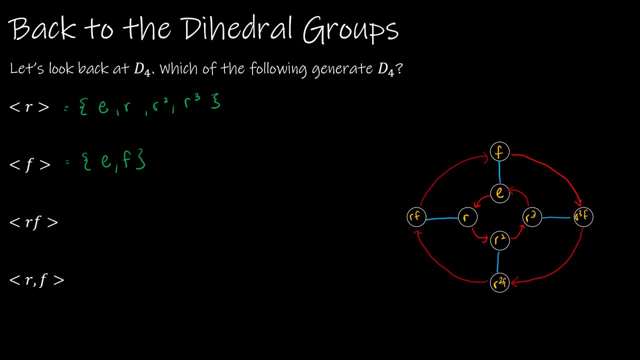 but it doesn't generate the entire set of D4. 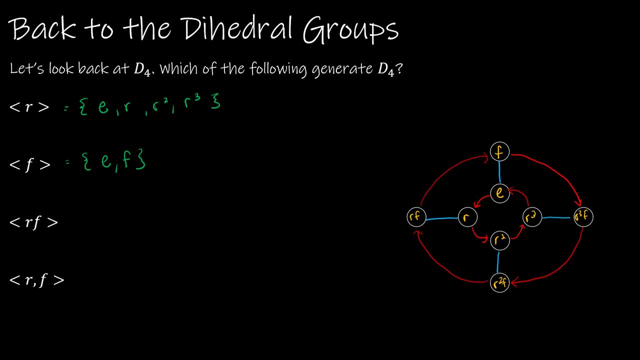 So, so far, we don't have any generators of D4. What about RF? Well, if I take RF and not do it, I get the identity. If I take RF and perform the action, so that's RF, I get RF. 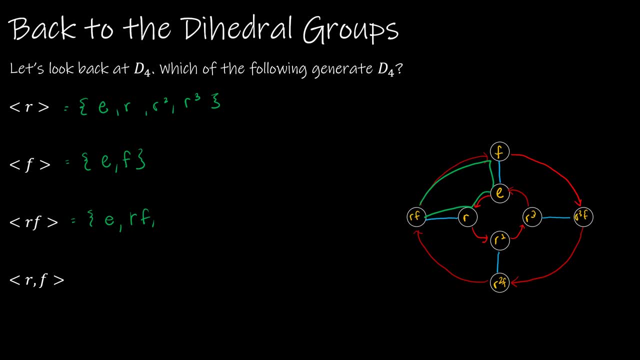 And if I do RF again, that would be RF. Notice I'm back at the identity. So again, it is a subgroup, but it is not the identity. So if I do RF again, that would be RF. Notice I'm back at the identity. 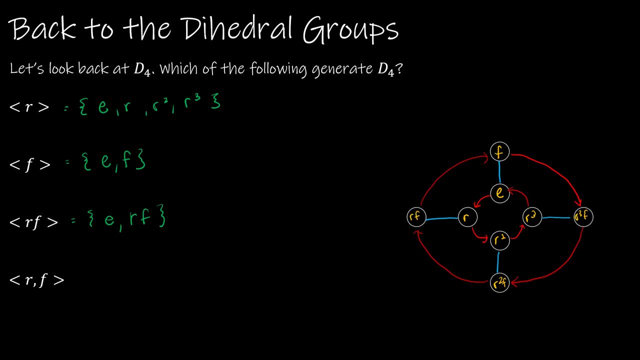 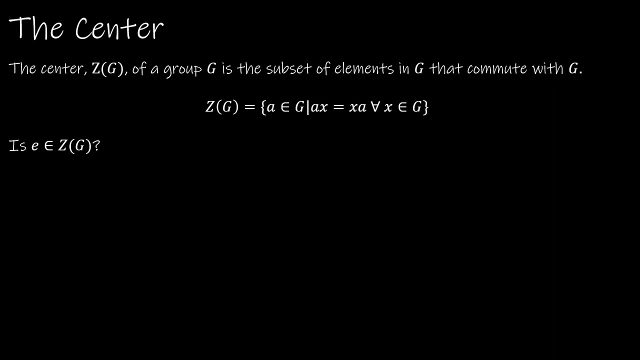 Now, I want you to notice the difference in notation between RF and R comma F. So if you have two elements, what we're saying is it's whatever's generated here, and whatever's generated here, and anything that you can generate with them together. So obviously, I already know that I can get E, R, R squared, R cubed, but with F, I can also get EF, which is F, RF, which is RF, R squared F, which is R squared F, R cubed F, which is R cubed F. And now we can see that we have actually generated the entire D4. So looking at R and F, a rotation and a reflection, I'm generating the entire set. And I'll leave it to you to see if there's any other combinations of rotations and reflections that generate D4. Let's talk now about the other subgroup that we wanted to talk about in this video, which is the center. So the center of a subgroup, I'm sorry, the center denoted Z of G of a group is the subset of elements in G that commute with G. So essentially, we're saying any element that's in G, where AX is equal to XA for every element of X in G. So it has to commute with all elements in G. So for instance, is E an element of the center? Well, it would make sense that EX is equal to XE for all Xs in G, because that is exactly what the 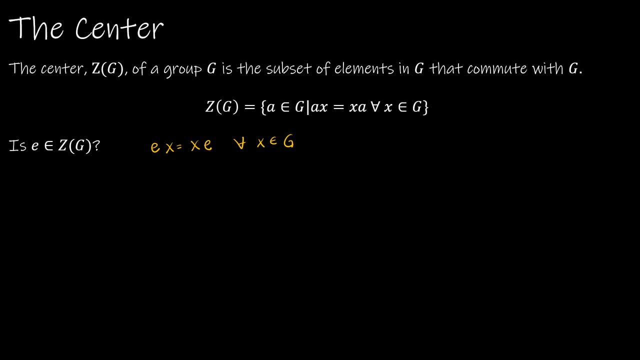 definition of X is. So that's exactly what the definition of X is. So that's exactly what the definition of the identity tells us is that EX is equal to XE for all X and G. So yes, the identity 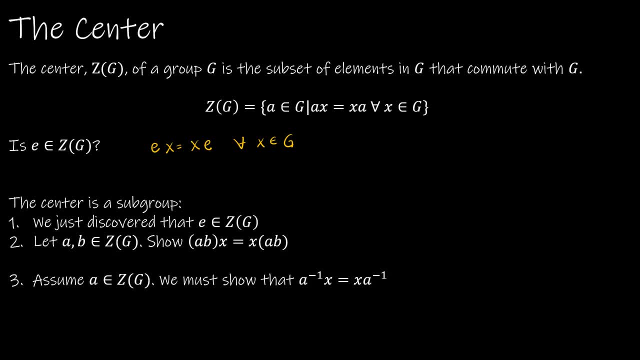 element will always be in the center. So is the center a subgroup? Yes, it is. We just discovered that the identity is an element of G. Now we're going to let A and B be in the center and show that ABX is equal to XAB. So that's fairly straightforward, because I knew that B would be on the center. But now we're in the center. Now I can see that XA is on the center. And that ABX is equal to XB, 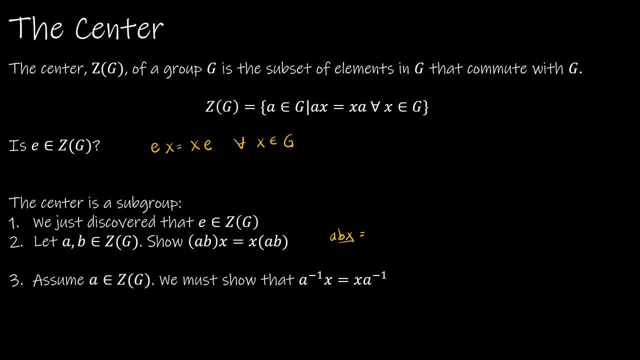 because XAB is union to G. So I know that ABX is equal to XAB. Now we're seeing these contrasting allezc values. And one more time, we're seeing that for this 계속 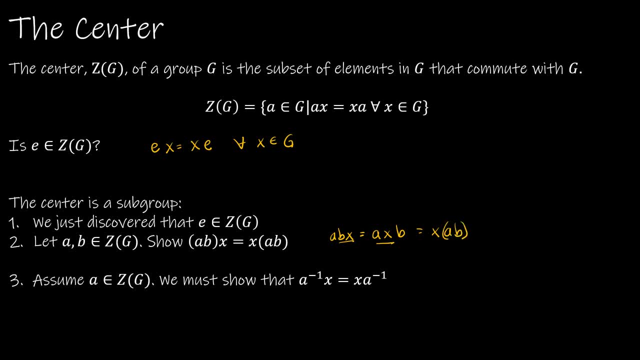 Thank you very muchằ� that this is equation the state of this value begins within this wave. 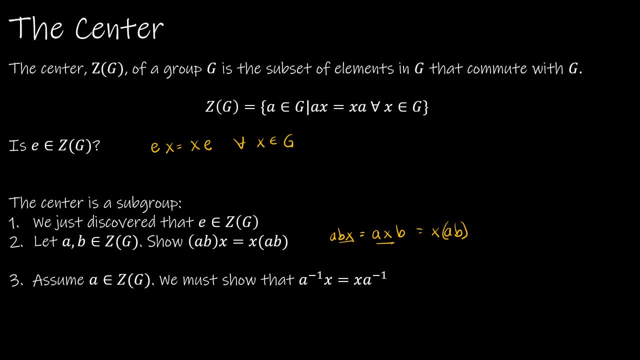 And by a final equation, we've already, it looks like we've reached the point where a B is x is equal to a, I'm sorry, xab. So that was fairly straightforward. Now let's assume that a is an element in the center. So we must show that a inverse is an element in the center. So again, fairly straightforward. If I start multiplying, I already know that ax is equal to xa. So let's multiply by the inverse on the left-hand side and multiply by the inverse on the right-hand side. So left-hand side, right-hand side. So what is that going to give me? These two cancel out. I get xa inverse. These two cancel out to give me the identity. So I get a inverse x. So I have just shown what I need to show. So it means it's all a inverse. So I have just shown what I need to show. 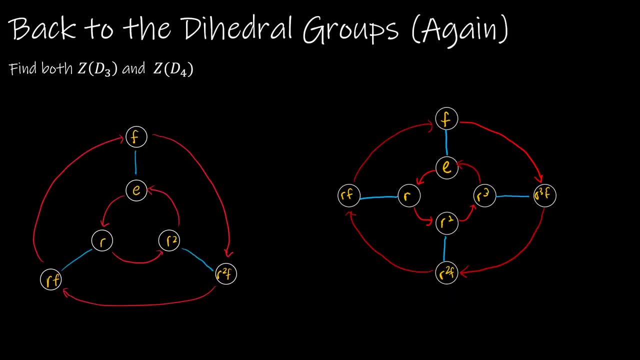 All of the requirements to be a subgroup. Since we've already refreshed our memory on the dihedral group D4, let's look at both D3 and D4 and see if we can determine the center of each group. So we already know that the center is going to include the identity, and that's for each group. 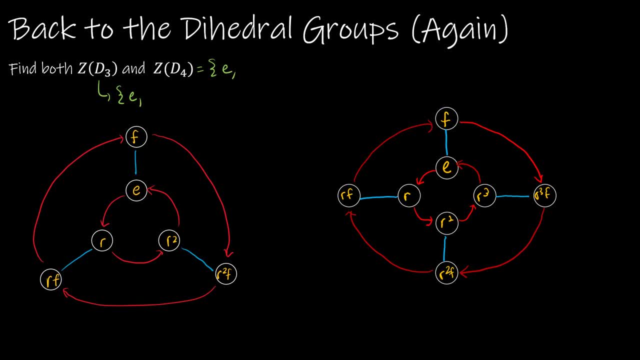 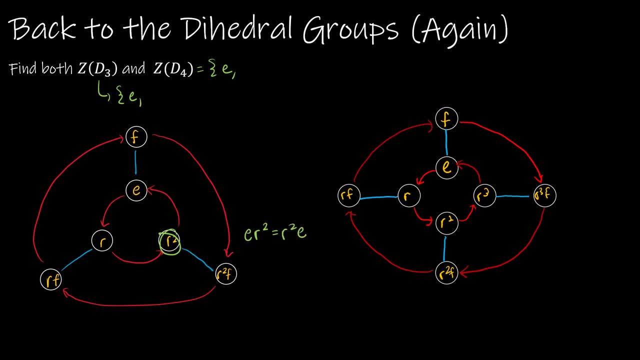 that e R squared would be the same as r squared e. We know that the identity doesn't do anything, and so whether I do perform the identity, whether I do nothing at the beginning or nothing at the end, it's not going to change. So we know for sure that's true. So now the question is, 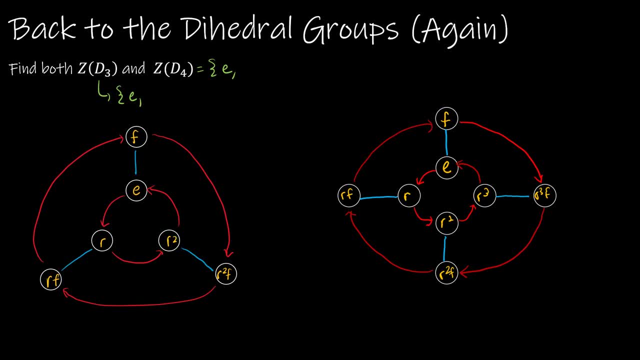 are there other elements that I can put out in either order so that commute with every other element of the group? So we could certainly do this the long way and start by checking R and saying, okay, does R commute with everything? Well, let's choose F and say, does RF equal FR? Well, RF gives me RF and FR gives me R squared F. So that's not the case. So in fact, I've shown that R is not in the center and that F is not in the center. Well, let's try R squared. Is R squared F the same as FR squared? So R squared F and then FR squared. Nope, not the case. So again, I've already now shown that R squared is not going 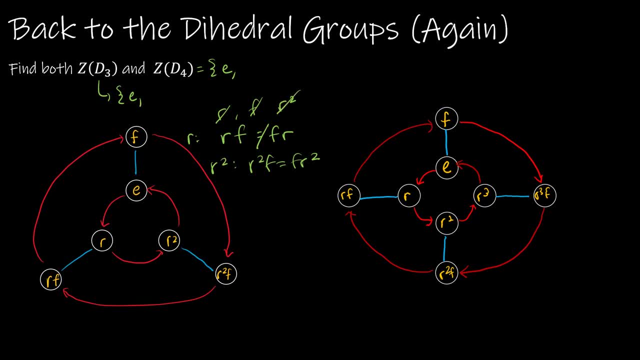 to commute with everything. Now, what about, what's the last one that I haven't tried? RF. I believe I've tried the rest of them. So RF, goodness gracious. Let me just try it again. RF. 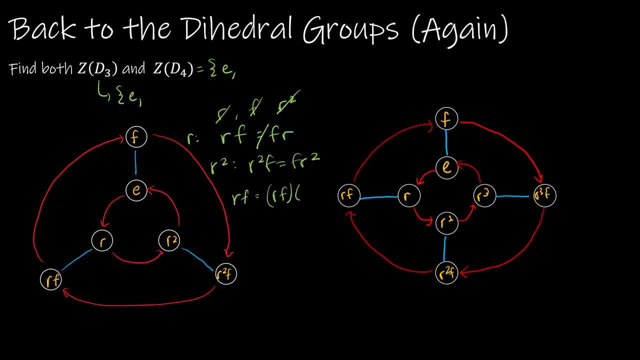 So is RF, and let's go ahead and knock out two birds with one stone, R squared F. Does that equal R squared F, RF? RF. Well, let's take a look. If I start at E, and I say RF, and then R squared F. Okay, I'm at R squared. Now let's try the other way. 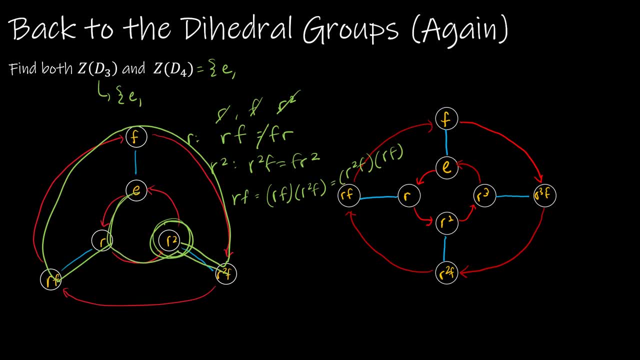 R squared F, and then RF. That leaves me with R. So again, those are not the same. So I've pretty much shown that the only thing in the center, the only element in the center of D3, 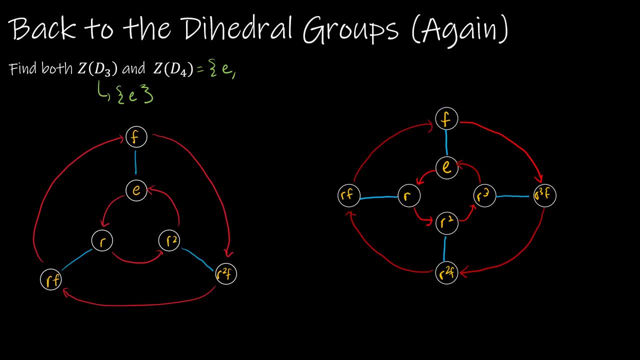 is the identity, because I've checked all of the other ones. Now, I can go through and do that as well for D4, but let's take a look at what we know about, say, RF. Essentially, what I know is that RF has to equal RF inverse in order for the element to commute, or the two elements, whether it's R and F. But we're just going to use R and F as an example. 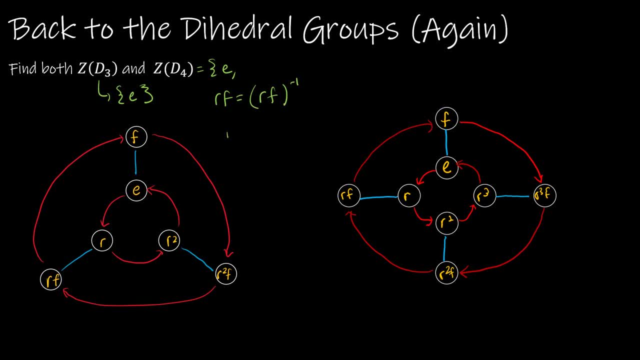 So for R and F to equal RF inverse, I need RF to equal, this is Sockshoe's property, F inverse R inverse. Well, what's the inverse of F? How do I undo F? I just do F again. So really, I'm looking at when does R arrive as the same as canvas under smoother points, which actions can 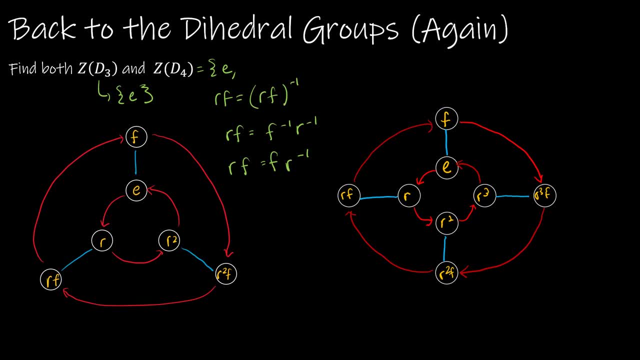 F do only chamber? This is exactly that problem that we learned using ajingles, and so這個 answering question will help us interpret it as well. So we need RF to equate RF inverse. And as our inverse well obviously the identity which we've already put in the 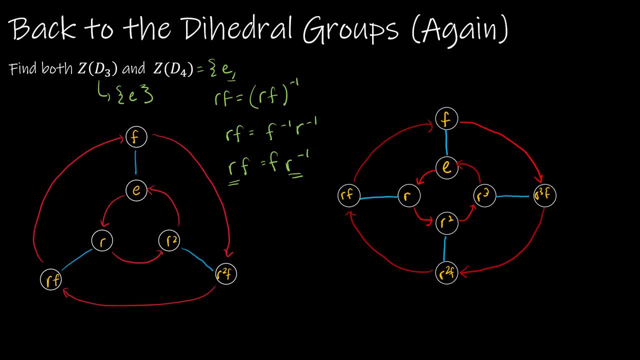 center but what about 4d for what about R squared does it make sense that R squared would be the same as R squared inverse so if I do R squared is that the same as moving twice in the opposite direction yes it is so let's just test it and make sure that works if I take F R squared would that be the same as R squared F so let's start at e F but take me to F and then R squared would take me to R squared F start at e do R squared and then F did it also take me to R squared F yes it did now we can check it against all of the elements but in fact this is going to work because you 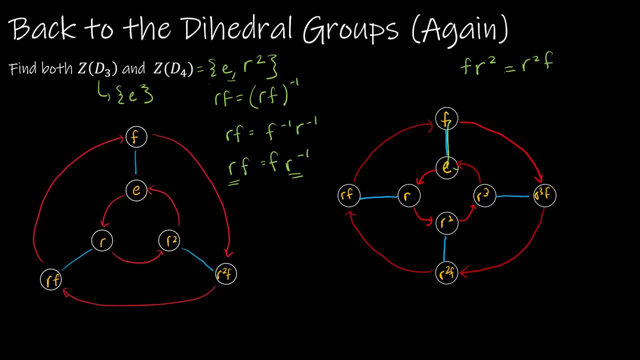 can see that the center of d3 is its own inverse so for d3 the center of d3 we have only the identity in the center of d4 we have the identity and R squared 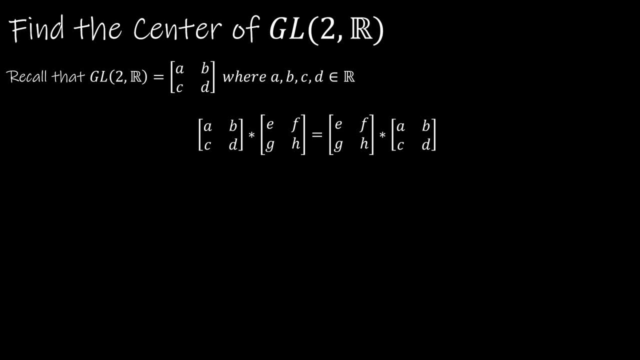 let's take a look at one more example of the center in this case we're looking at the general linear group 2 R remember that just tells me that I'm looking at a 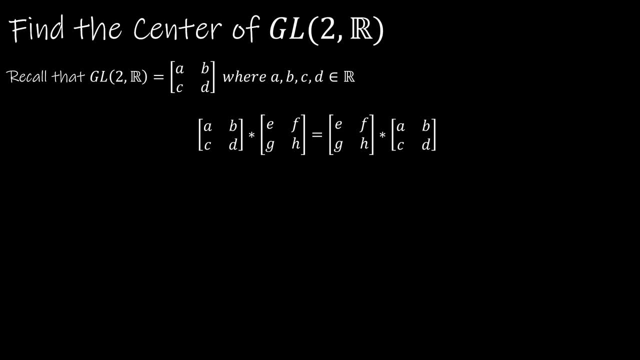 2 by 2 matrix where all entries are real numbers and what we're trying to do is find what's going to be the format of the 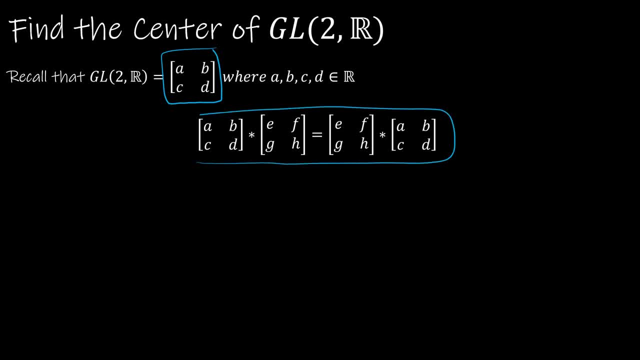 matrix so that this equation is true well we know that matrices are tricky because matrix matrix multiplication is not commutative so what I'm asking you to do is find what elements are in fact commutative well we know 1 and that's 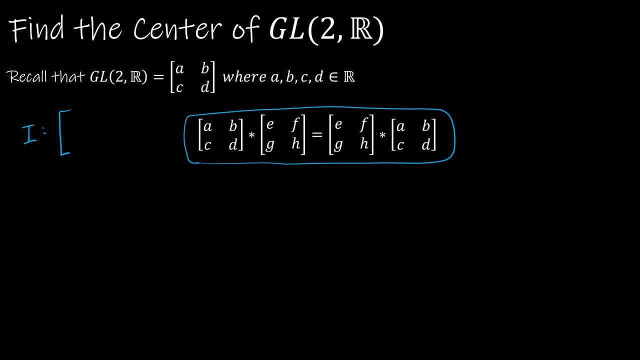 the identity because we always know that the center is going to include the identity and in that case that's 1 0 0 1 so let's go off of that a little bit and say okay let's 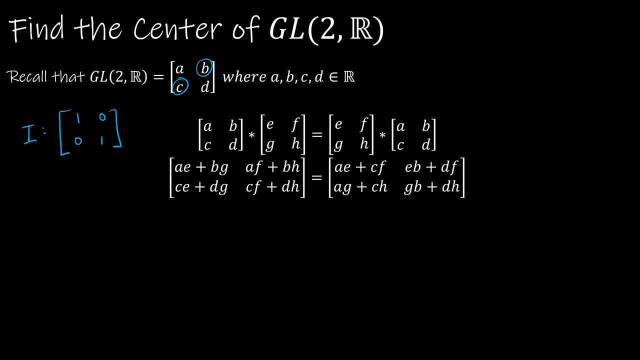 let B and C be zeros. So when I do the matrix multiplication, I'm going to let any value that includes B or C be zero. So that's going to get rid of BG and CE and BH and CF and CF and CH and EB and GB. Well, that makes things a lot easier because now all I need is for AE to equal AE, 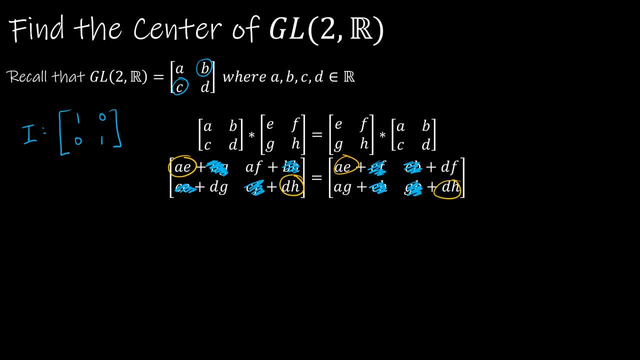 done, for DH to equal DH, done, to let AF equal DF, not done, and let DG equal AG, not done. But by some simple math, I can say that if A is equal to B, 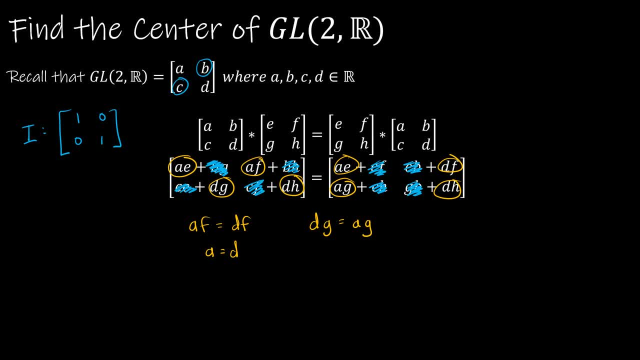 then I can say that if B is equal to B, then I can say that if B is equal to B, then I can say that if B is equal to B, to D and if D is equal to a then this is going to work out okay so what is going 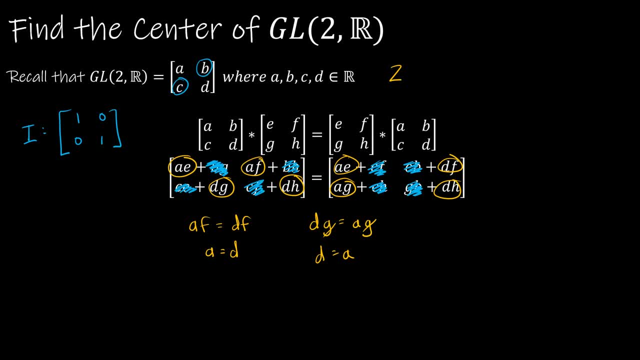 to be the center well the center of the general linear group 2 oops 2r is going to be all matrices in the form a 0 0 a for all a in R again because we've let a equal to D so as long as a is equal to D so the first diagonal is the same and the second diagonal is zeros we're going to be able to commit up next 1 will take a look at cyclic groups and their properties.